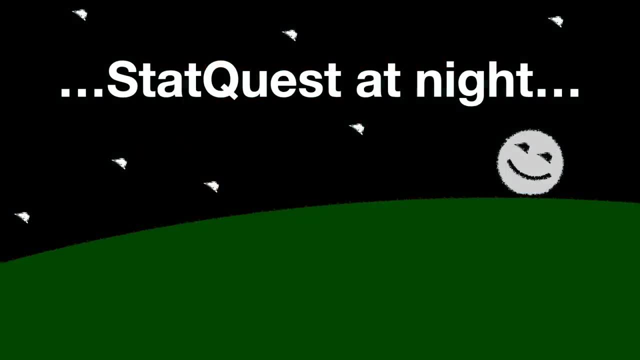 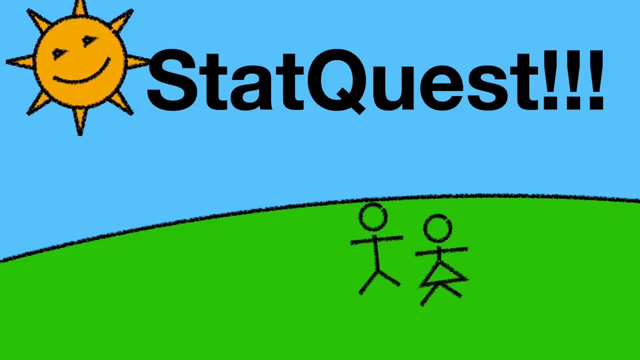 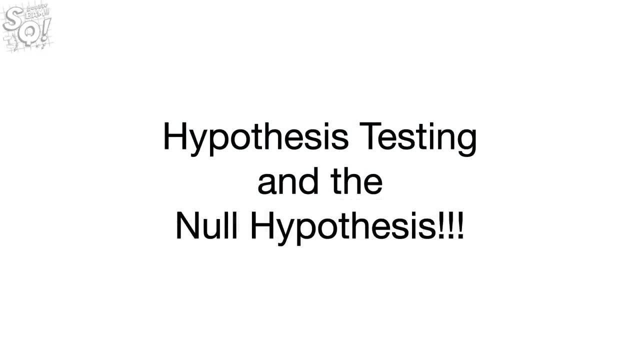 StatQuest in the morning. StatQuest at night, StatQuest in the afternoon. it's all right, StatQuest. Hello, I'm Josh Starmer and welcome to StatQuest. Today we're going to talk about hypothesis testing and the null hypothesis. I'm not going to name names, but imagine there was a virus. 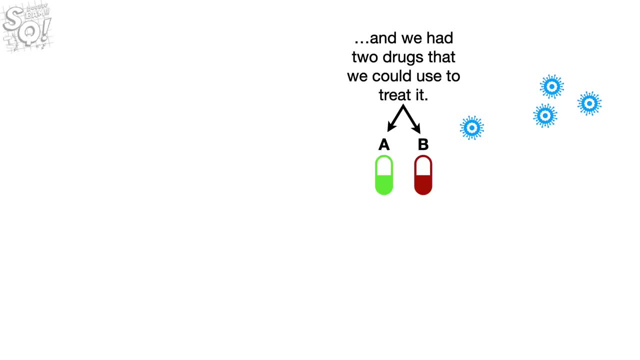 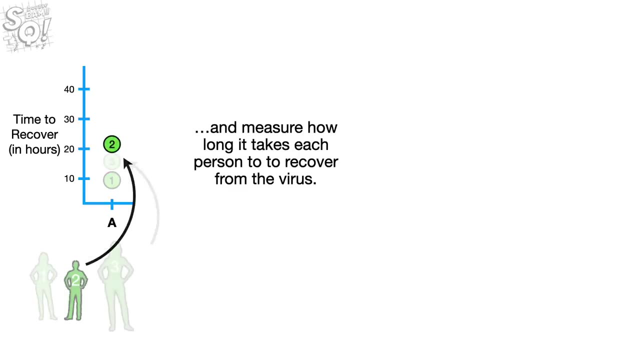 and we had two drugs we could use to treat it. So we give drug A to three people and measure how long it takes each person to recover from the virus. The first thing we notice is that not everyone recovered in the exact same amount of time. Person number one recovered the fastest. 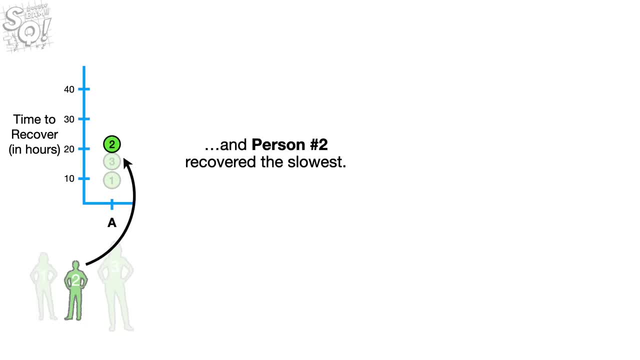 and person number two recovered the slowest. It's possible that person number one either recovered the fastest or the slowest. Person number one eats healthy food and exercises and already has a strong immune system and that helped them recover quickly, And maybe person number two doesn't get as much exercise, Or 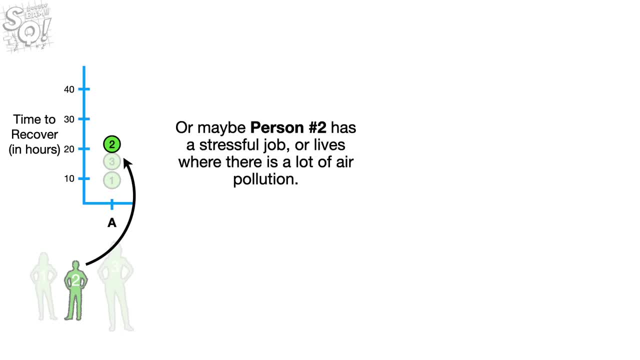 maybe person number two has a stressful job or lives where there is a lot of air pollution. The point is is that even though all three people had the same virus and took the same drug, they did not all recover in the exact same amount of time, And that might be due. 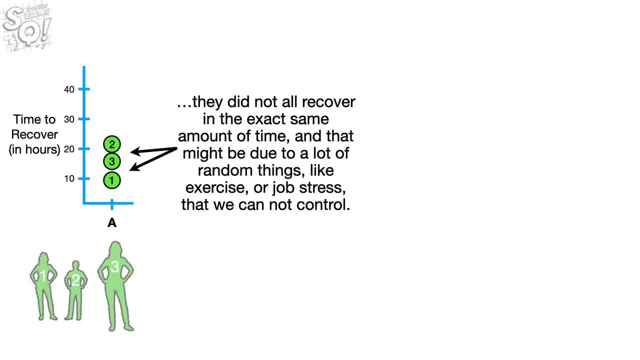 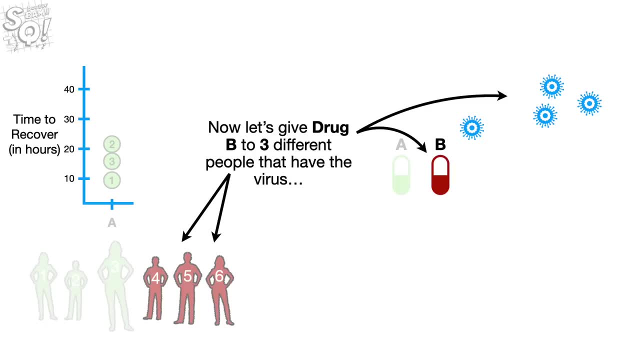 to a lot of random things like exercise or job stress that we cannot control. Now let's give drug B to three different people that have the virus and measure how long it takes them to recover. Again, we see that even though three people had the same virus and took the same drug, they did not all recover in the exact same amount of time. 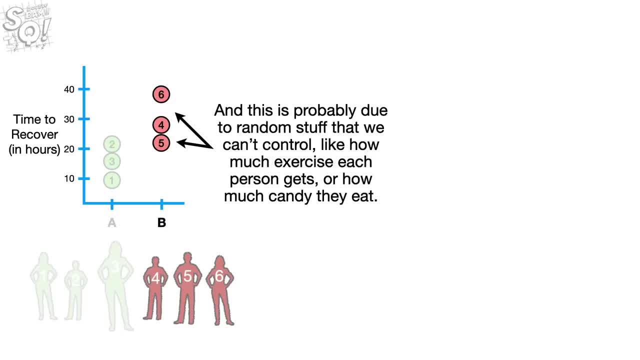 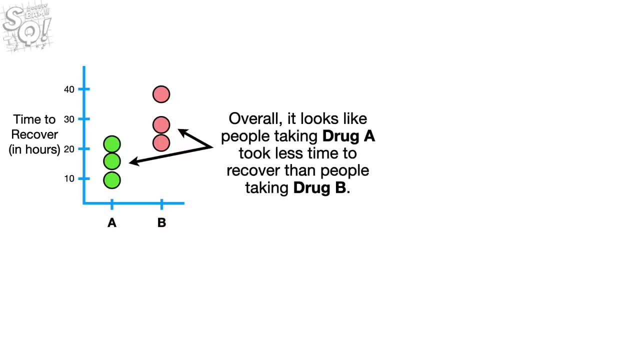 And this is probably due to random stuff that we can't control. but we can't control the virus, So we can measure how long it takes them to recover, Like how much exercise each person gets or how much candy they eat. Overall, it looks like people taking drug A took less time to recover than people taking drug B. 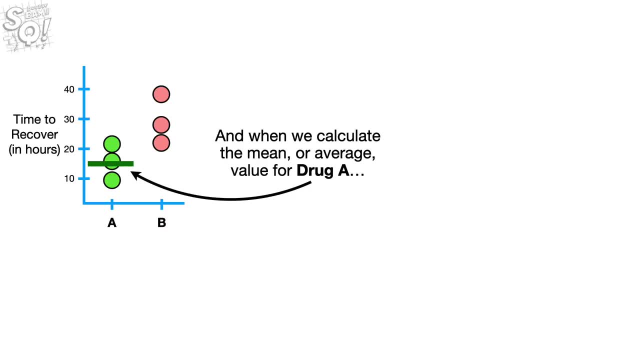 And when we calculate the mean or average value for drug A and the mean value for drug B, we see that on average there is a 15-hour difference between drug A and drug B. So after seeing this preliminary data, it might seem reasonable to form the following hypothesis. 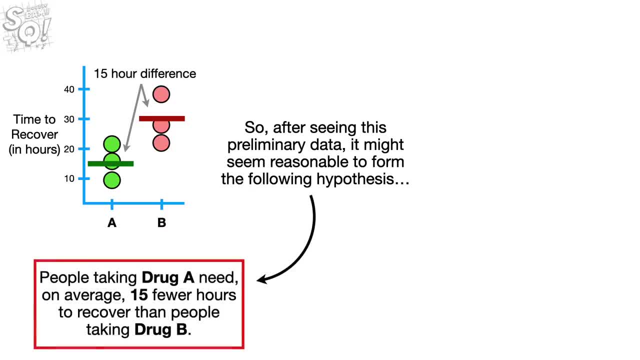 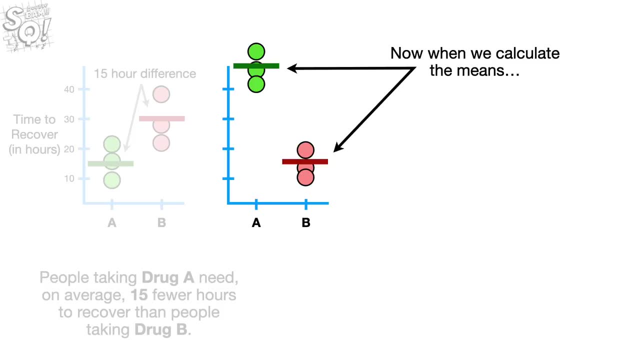 People taking drug A need, on average, 15 fewer hours to recover than people taking drug B, And now that we have this hypothesis, we can test it by repeating the experiment. Now, when we calculate the means, we see that, on average, people taking drug A need 15 fewer hours. 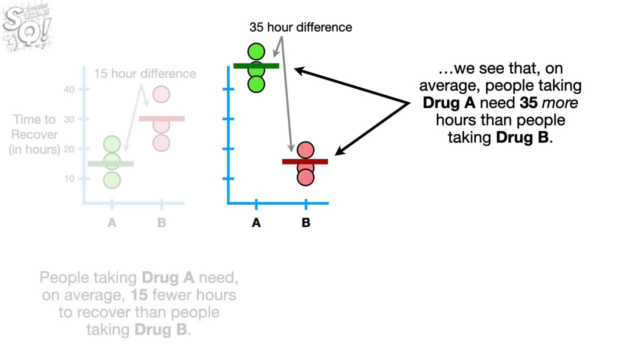 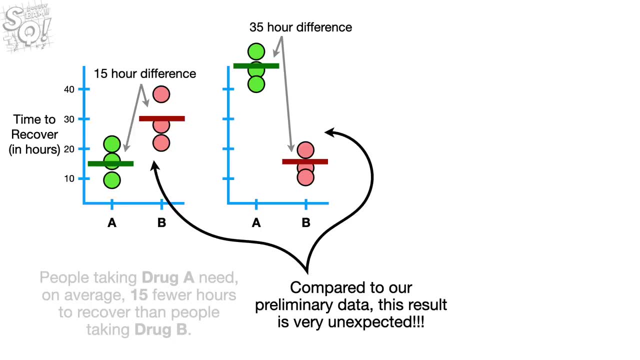 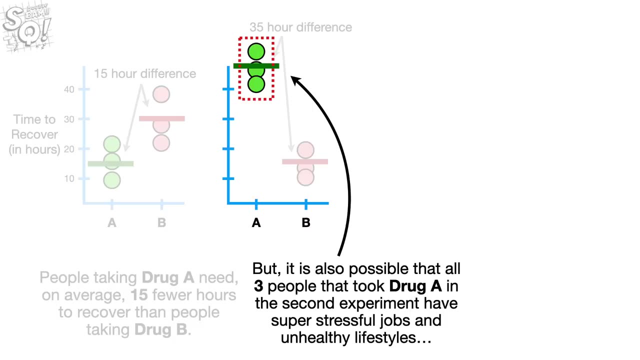 to recover than people taking drug B. Compared to our preliminary data, this result is very unexpected. In fact, it is the opposite of the original hypothesis. But it is also possible that all three people that took drug A in the second experiment have super stressful jobs and unhealthy lifestyles. 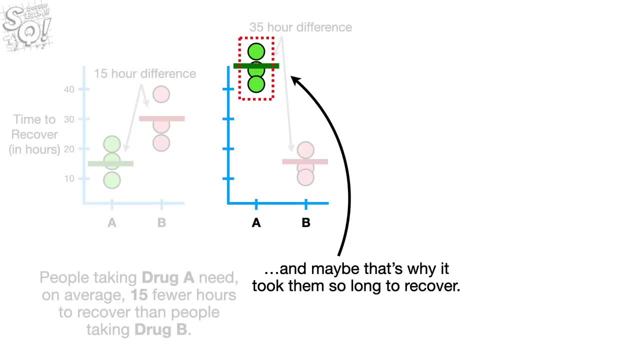 And maybe that's why it took them so long to recover. And maybe everyone taking drug B was well-rested and super healthy to begin with And maybe that's why they recovered so quickly. But it is also possible that we mislabeled drug A and drug B and did the wrong experiment. 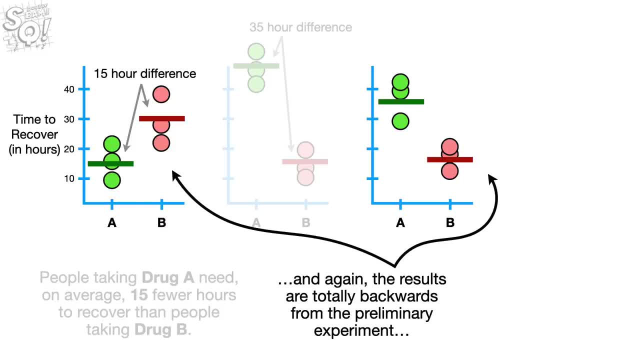 So we repeat the experiment And again the results are totally backwards from the preliminary experiment and totally backwards from the hypothesis that we made. So again, just to make sure we didn't mislabel things, we redo the experiment And again these results are the opposite of the original hypothesis. 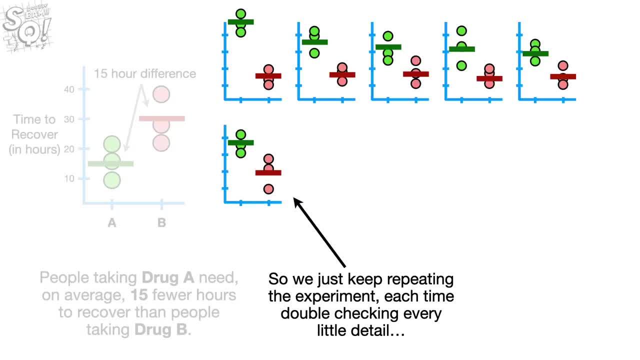 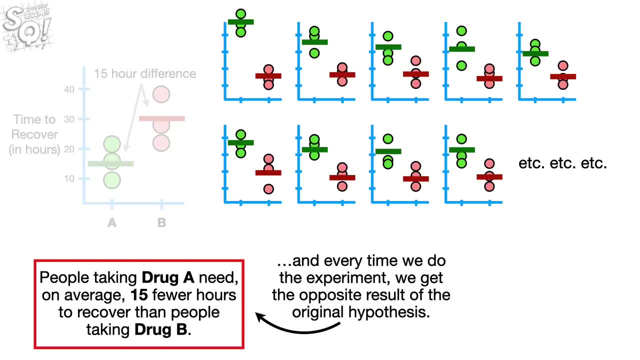 So we just keep repeating the experiment, each time double-checking every little detail, And every time we do the experiment we get the opposite result of the original hypothesis. So after doing all of these experiments, we get the opposite result. all of these repeated experiments where we double-checked every little. 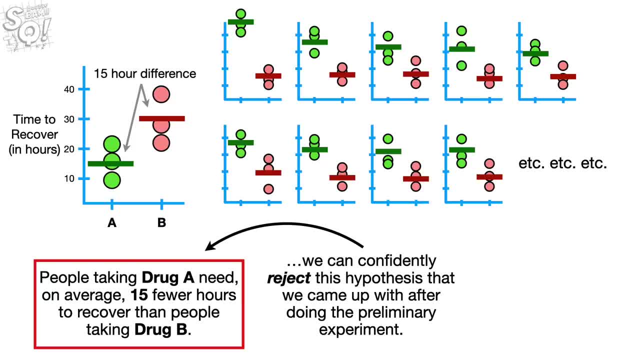 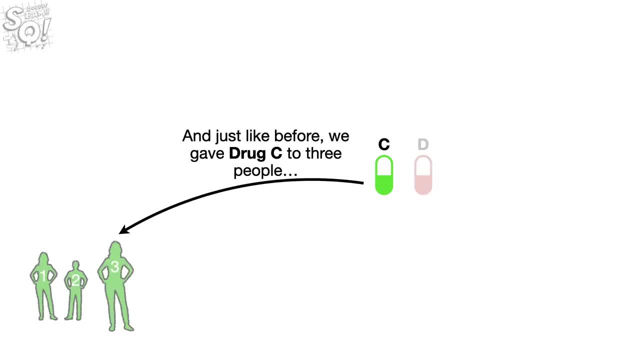 step we can confidently reject this hypothesis that we came up with after doing the preliminary experiment Bam. Now let's imagine we had two more drugs, C and D, And, just like before, we gave drug C to three people and measured how long it took each. 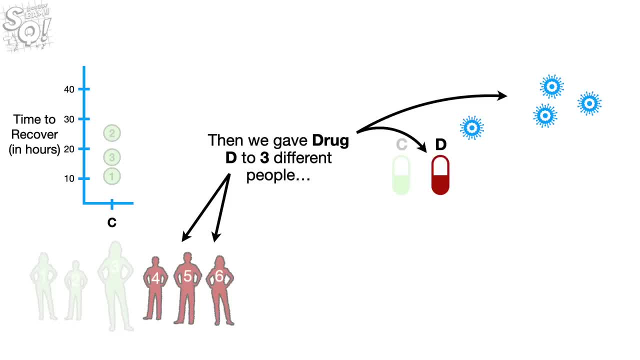 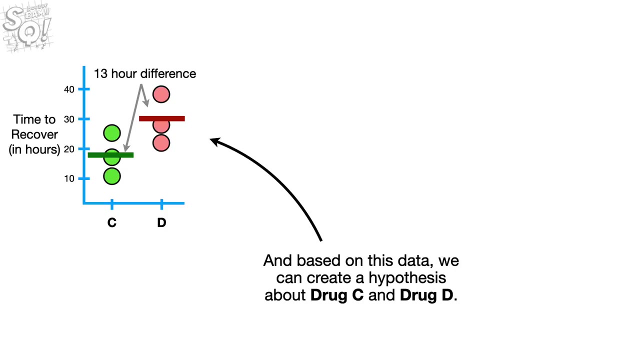 person to recover from the virus. Then we gave drug D to three different people and measured how long it took them to recover from the virus And based on this data we can create a hypothesis about drug C and drug D. People taking drug C need, on average, 13 fewer hours. 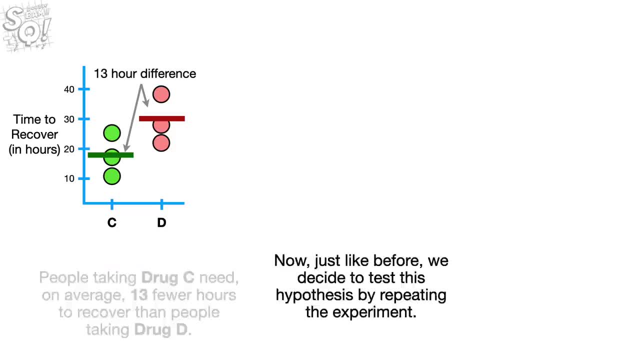 to recover than people taking drug D. Now, just like before, we decide to test this hypothesis by repeating the experiment. Only this time, instead of getting something that's the exact opposite of what we expected, we get something that is only slightly different In this. 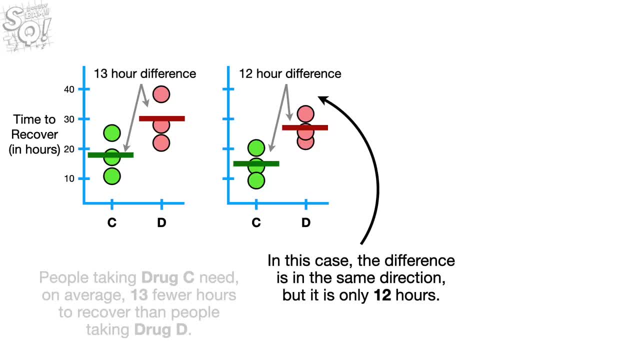 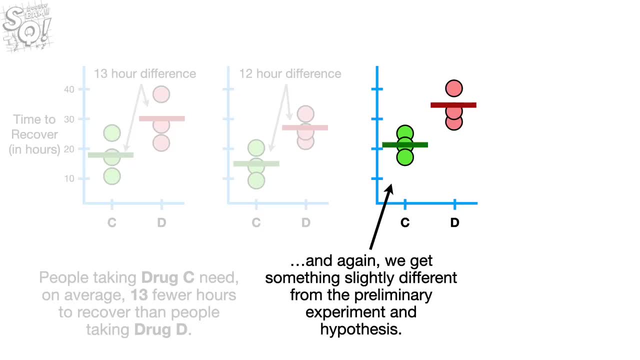 case, the difference is in the same direction, but it is only 12 hours. Then we repeat the experiment again and again. we get something slightly different from the preliminary experiment, but it is only 13.5 hours. The good news is that we probably didn't mislabel the drug like we did last time. 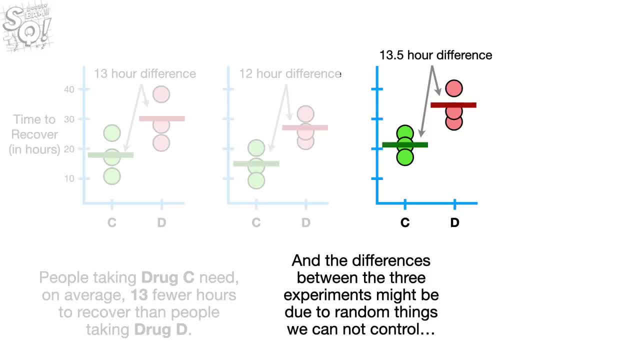 And the differences between the three experiments might be due to random things we cannot control, Like maybe these people exercised a lot and had relatively healthy diets compared to these people who took longer to recover. But regardless, the hypothesis says that people taking drug C needed 13 fewer hours to recover. 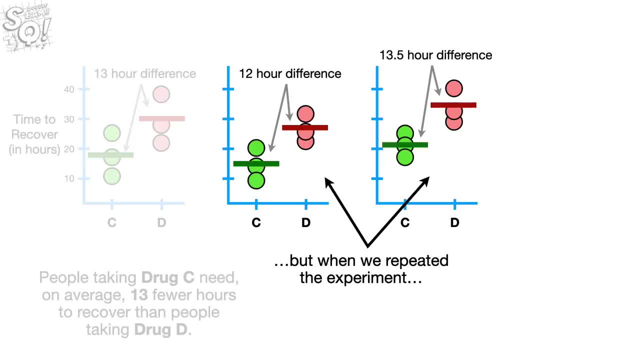 But when we repeated the experiment, the first replicate said the difference between averages was 12,, which is different from the hypothesis, And the second replicate said the difference was 13.5, which is also different from the hypothesis. And, let's be honest, The only reason, the 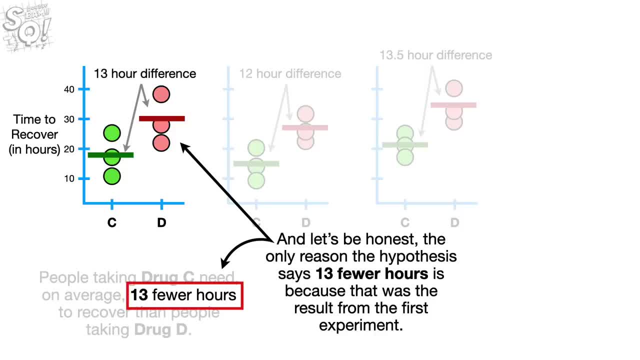 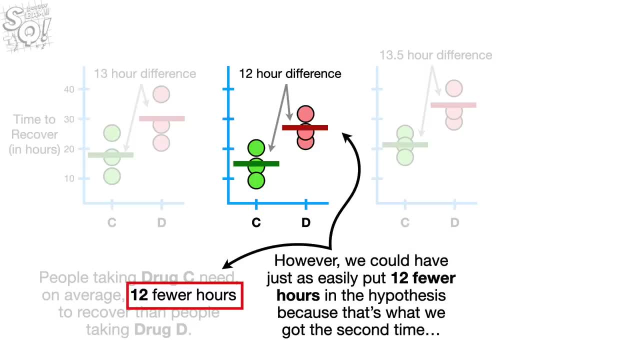 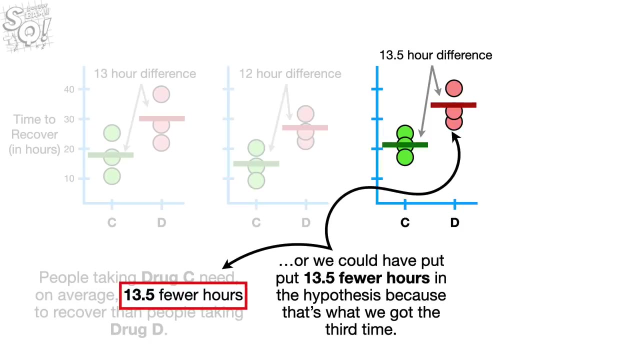 hypothesis says 13 fewer hours is because that was the result from the first experiment. However, we could have just as easily put 12 fewer hours in the hypothesis, because that's what we got the second time. Or we could have put 13.5 fewer hours in the hypothesis, because that's what we got the third. 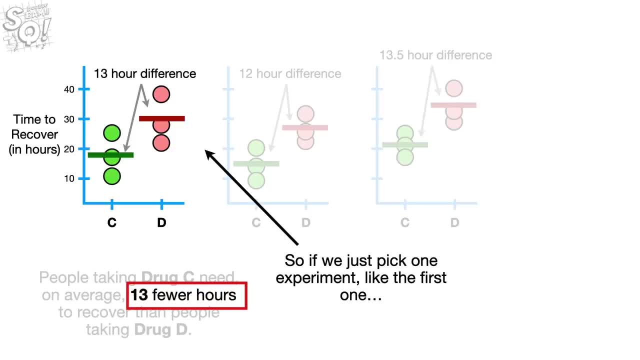 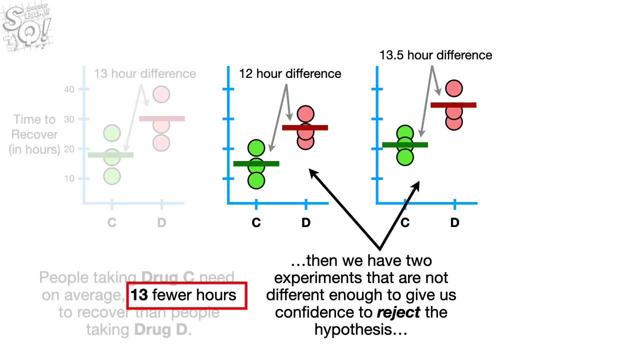 time. So if we just pick one experiment like the first one and use that to define the hypothesis, then we have two experiments that are not different enough to give us confidence to reject the hypothesis, But because there is just as much data suggesting that the difference is 12. 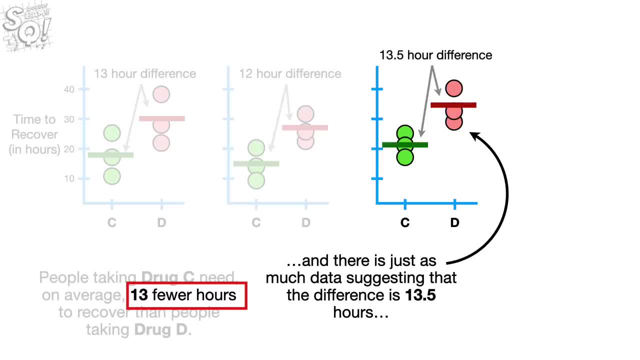 hours and there is just as much data suggesting that the difference is 13.5 hours. these experiments don't make us super confident that the hypothesis of 13 fewer hours is correct. Again, maybe drug A reduces recovery by 13 fewer hours, but maybe it reduces. 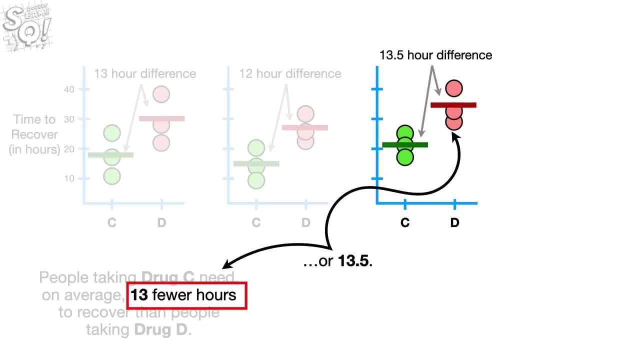 recovery by 12 hours or 13.5.. Because the results from the repeated experiments are not different enough to cause us to reject the hypothesis, and because they don't convince us that the hypothesis is correct either, the best we can do is fail to reject the hypothesis. 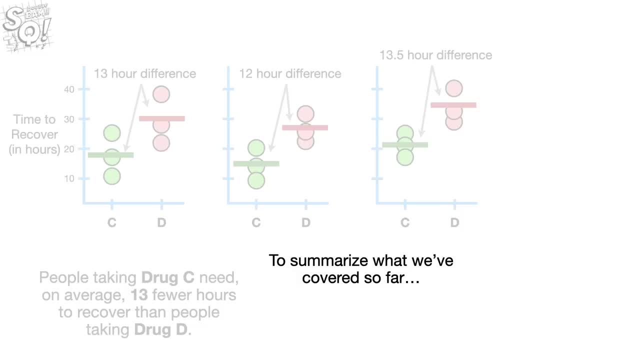 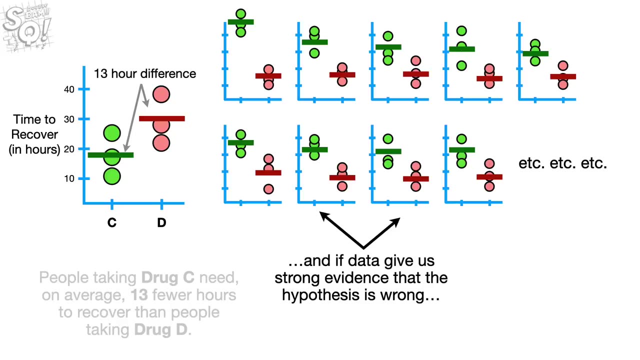 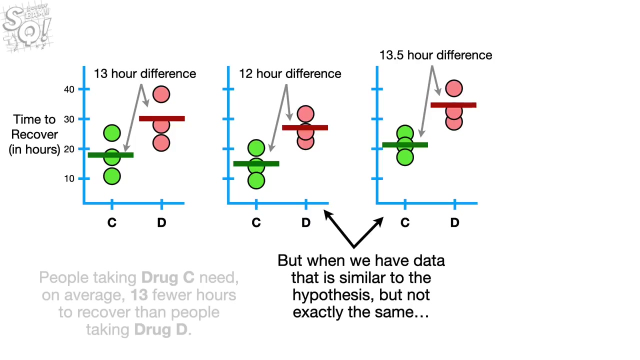 Small bam To summarize what we've covered so far. we can create a hypothesis and if data gives us strong evidence that the hypothesis is wrong, then we can reject the hypothesis. But when we have data that is similar to the hypothesis but not exactly the same, 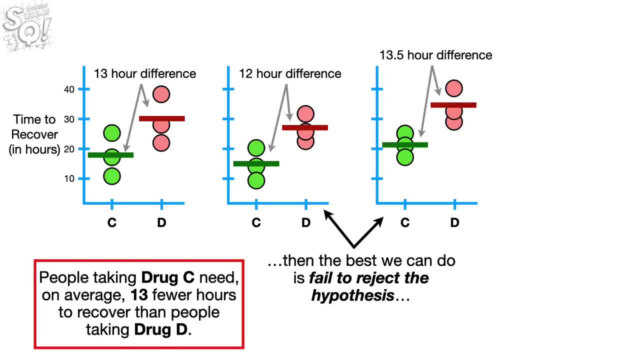 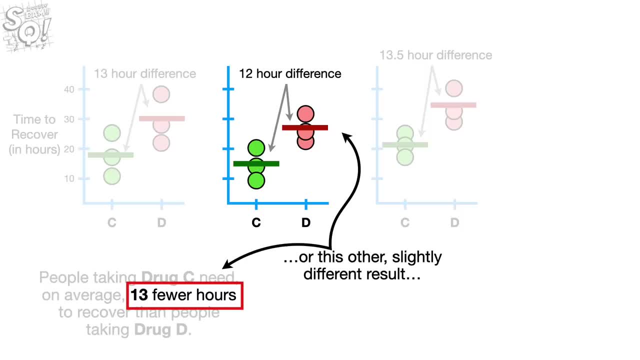 then the best we can do is fail to reject the hypothesis, Because it's unclear if the hypothesis should be based on this result or this other slightly different result, or this result or any other possible outcome- Double bam. Now let's take a closer look at the hypothesis itself. You may remember that the only reason 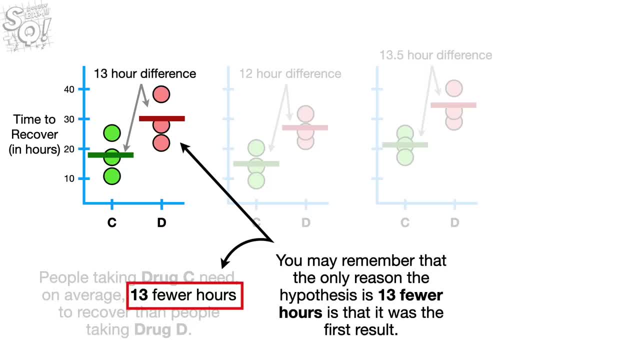 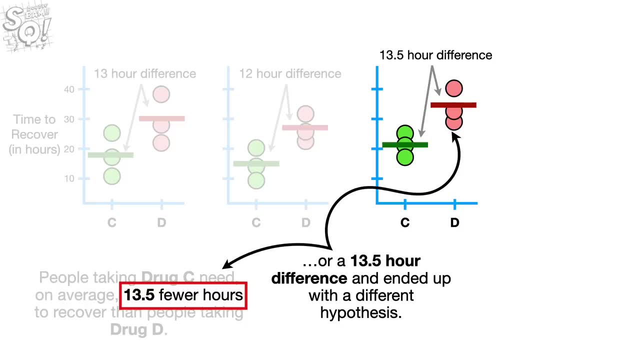 the hypothesis is 13 fewer hours is that? it was the first result, But we could have just as easily gotten a 12 hour difference or a 13.5 hour difference And ended up with a different hypothesis. And if 12 and 13.5 are reasonable hypotheses, then so is 12.25 or 13.1.. 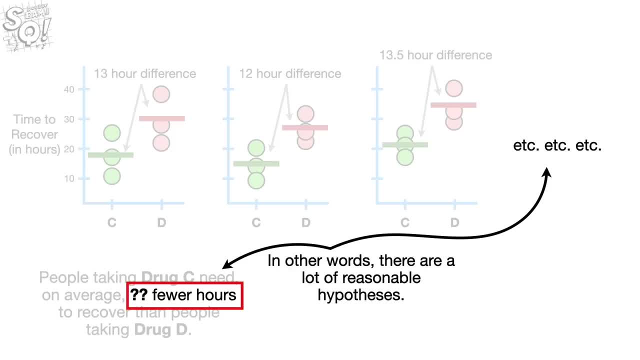 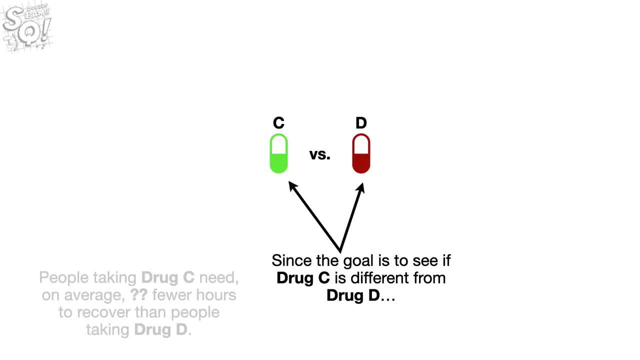 In other words, there are a lot of reasonable hypotheses. How do we know which one to test? Since the goal is to see if drug C is different from drug D, we simply test to see if there is no difference between drug A and drug B. 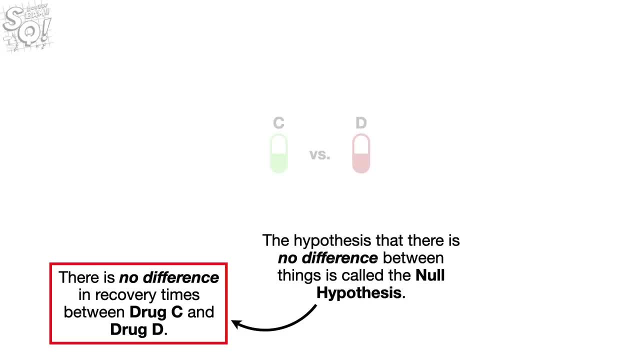 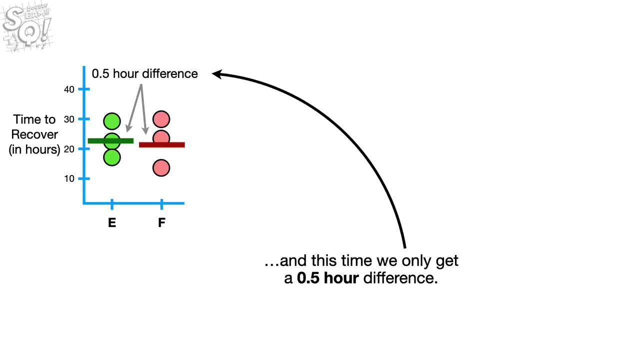 Oh no, it's the dreaded terminology alert. The hypothesis that there is no difference between things is called the null hypothesis. So let's take a look at two examples of the null hypothesis in action. Now imagine we are testing two new drugs, E and F, And this time we only get a 0.5 hour. 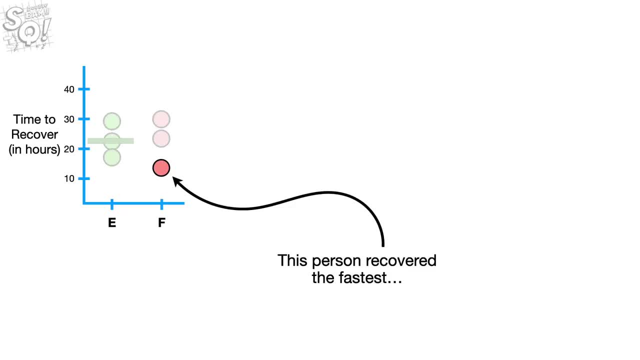 difference. This person recovered the fastest, but it is easy to imagine that if they had exercised a little less or had a slightly worse diet, then they might have taken a little longer to recover. Likewise, if this person was just a little healthier to begin with, then they might have. 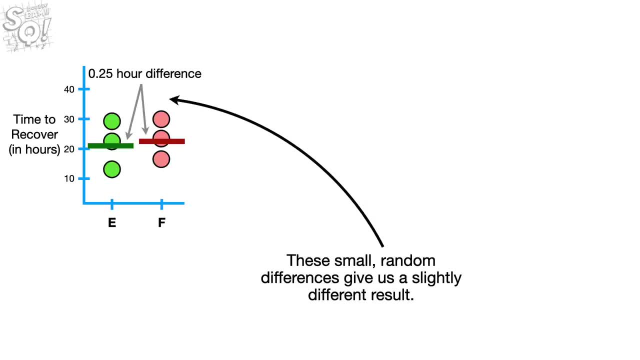 recovered a little more quickly. These small, random differences give us a slightly different result. Now, instead of drug F being 0.5 hour, we get a 0.5 hour difference. Now, instead of drug F being 0.5 hour, we get a 0.5 hour difference. 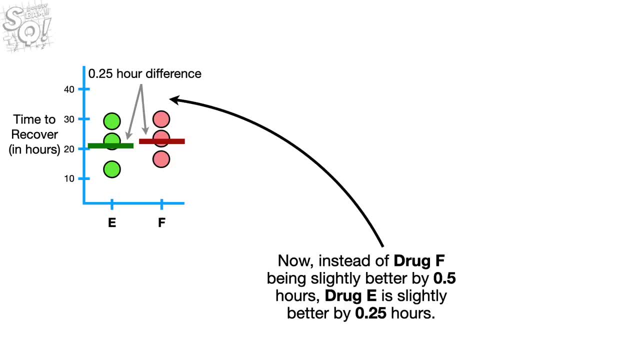 Now, instead of drug F being 0.5 hour, we get a 0.5 hour difference. Now if, the drug F being slightly better by 0.5 hours, drug E is slightly better by 0.25 hours. 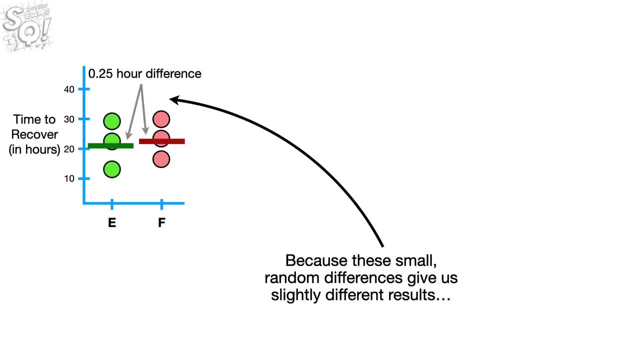 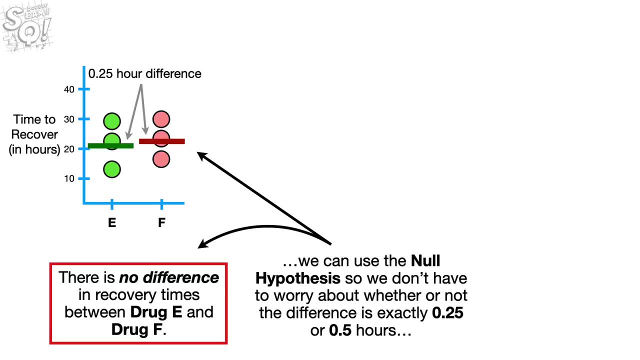 Because these small random differences give us slightly different results, we can use the null hypothesis, so we don't have to worry about whether or not the difference is exactly 0.25 or 0.5 hours. Instead, we simply see if the data convinces us to reject the hypothesis that there is. 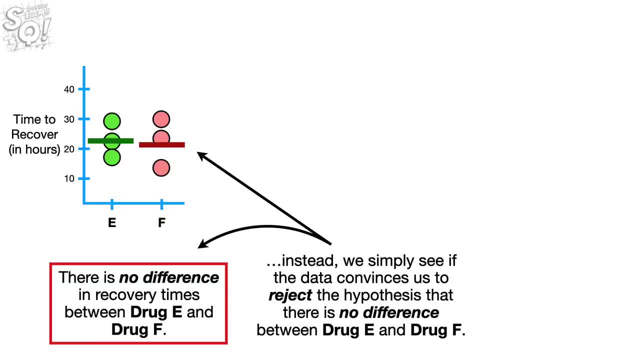 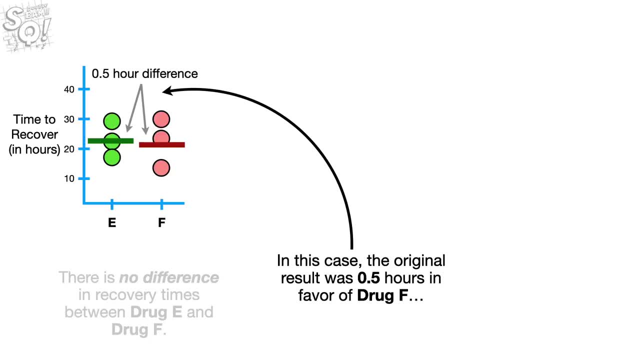 no difference between drug E and drug F In this case. the original result was 0.5 hours in favor of drug F, But small random things could have easily changed the result to be a 0.25 hour difference in favor of drug E, And thus the data does not overwhelmingly. 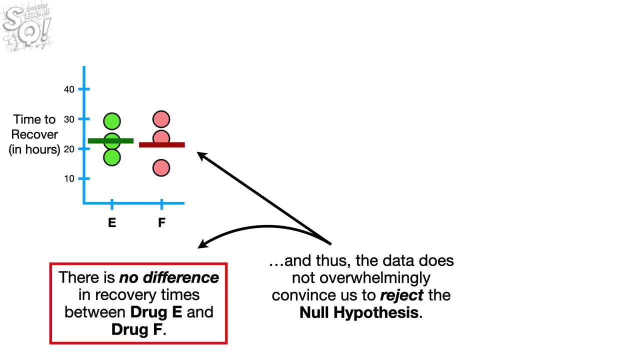 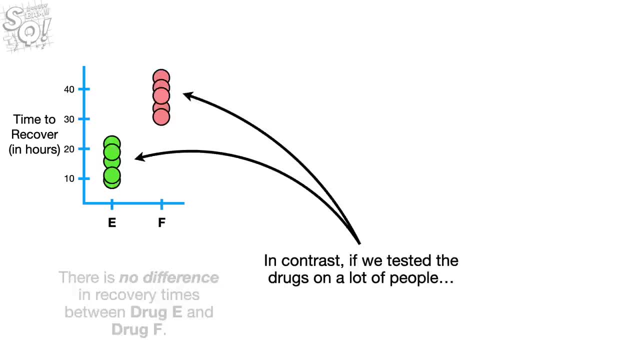 convince us to reject the null hypothesis. So we fail to reject the null hypothesis that there is no difference between the drugs. In contrast, if we tested the drugs on a lot of people and little random things would not change the results very much, then we. 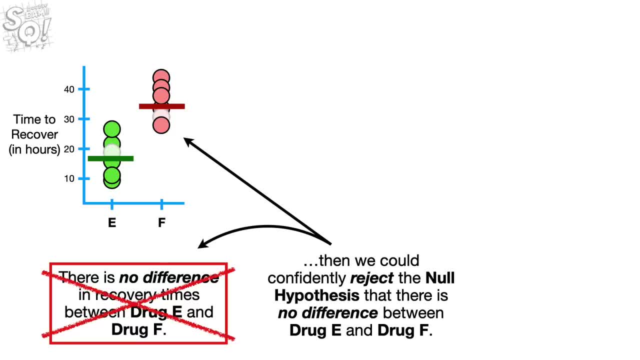 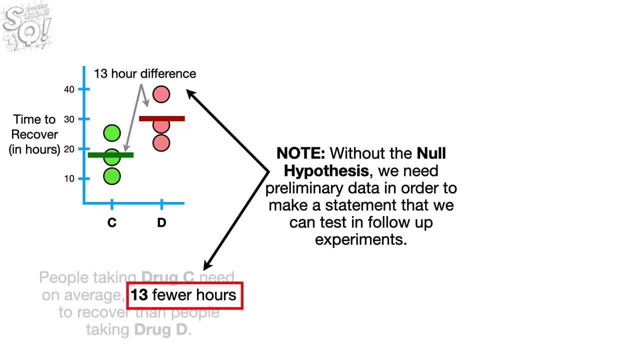 could confidently reject the null hypothesis that there is no difference between drug E and drug F Bam. Without the null hypothesis, we need preliminary data in order to make a statement that we can test in follow-up experiments. This is because we don't know if we should. 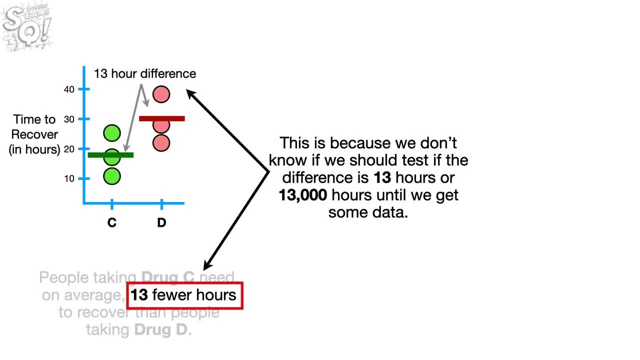 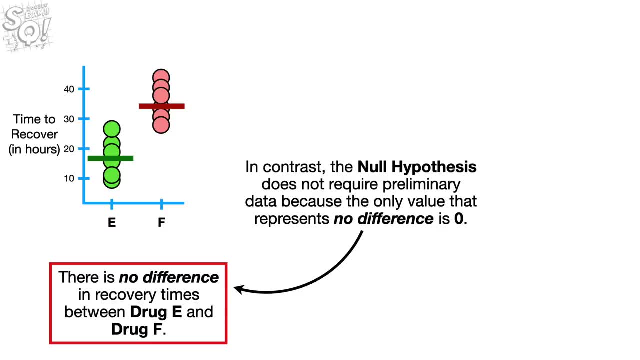 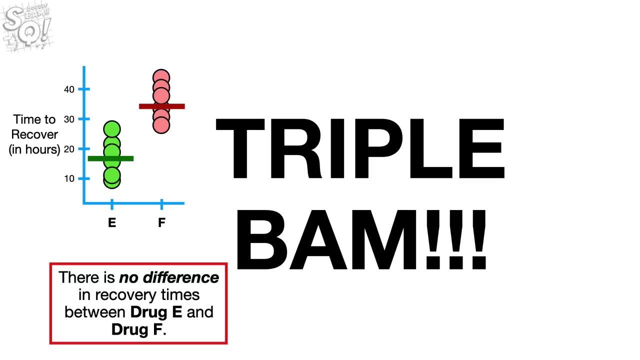 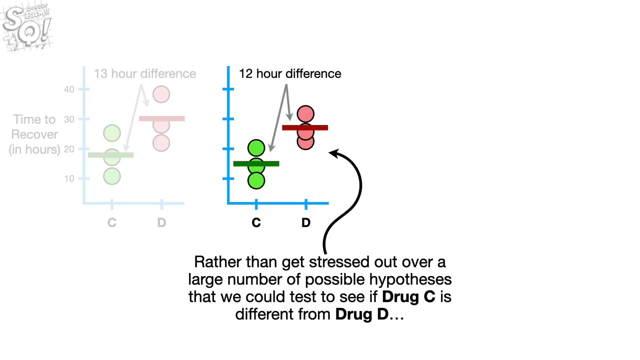 test if the difference is 13 hours or 13,000 hours until we get some data. In contrast, the null hypothesis does not require preliminary data because the only value that represents no difference is 0.. 3. RIPPLE BAM, In summary, rather than get stressed out over a large number of possible hypotheses, that 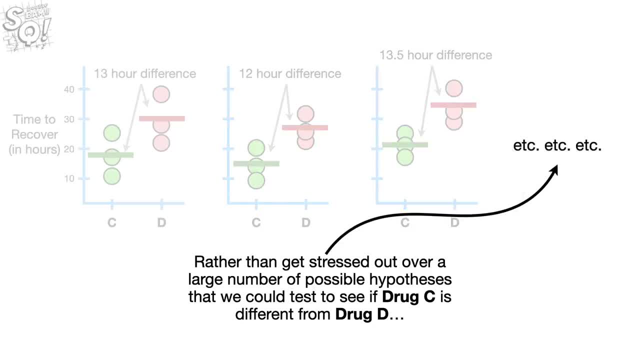 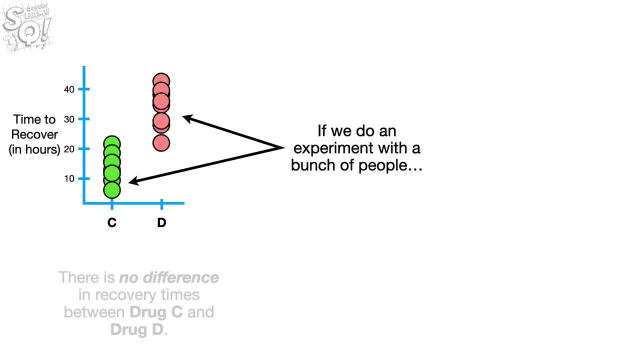 we could test to see if drug C is different from drug D. we use the null hypothesis to determine if there is a difference. If we do an experiment with a bunch of people, and a lot more people taking drug C had shorter recovery times than people taking drug D. 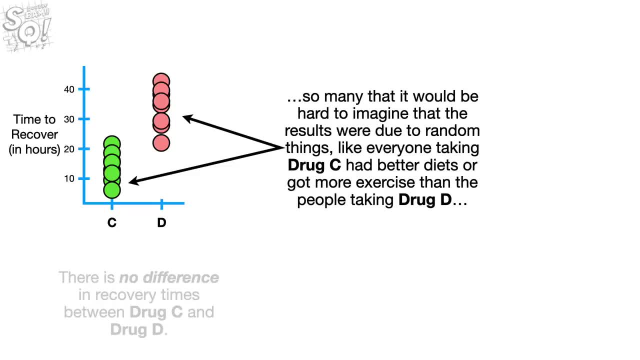 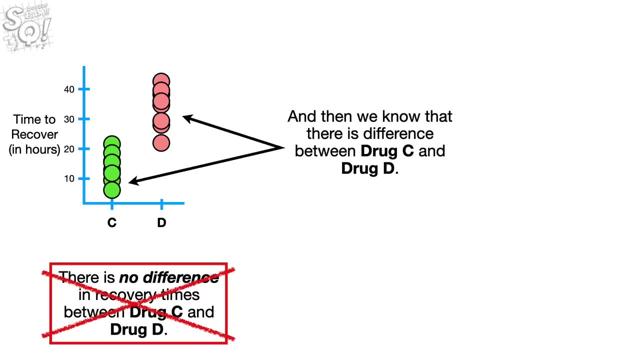 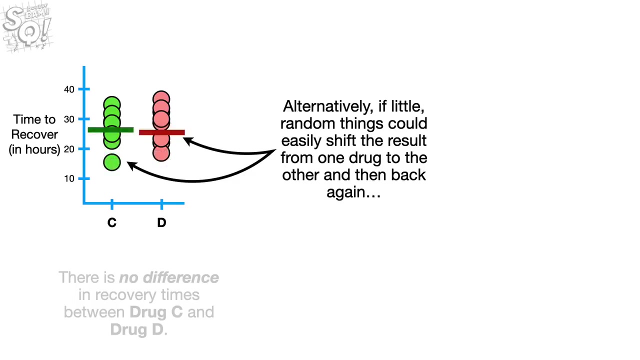 so many that it would be hard to imagine that there would be a difference between drug D and drug E. Then we could reject the null hypothesis And then we know that there is a difference between drug C and drug D. Alternatively, if little random things could easily shift, 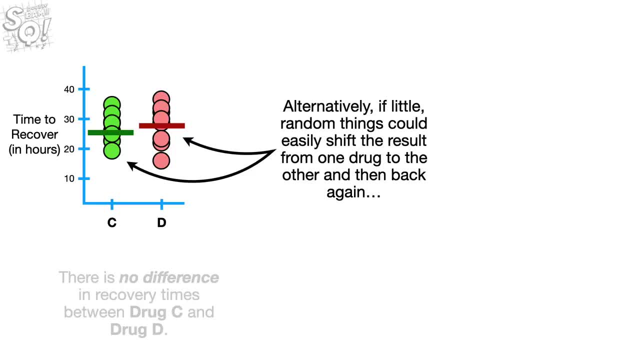 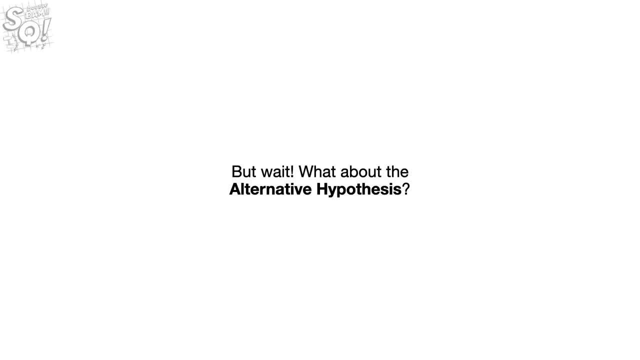 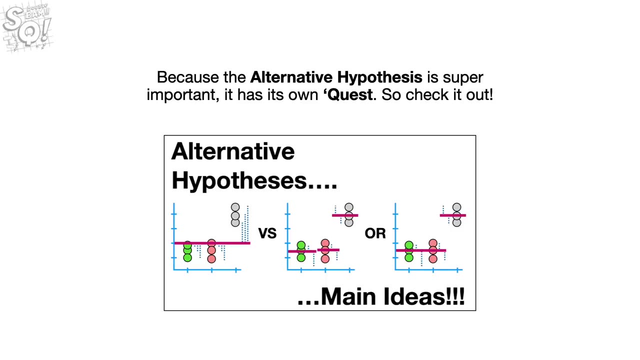 the result from one drug to the other and then back again. then we would fail to reject the null hypothesis BAM. But wait, what about the alternative hypothesis? Because the alternative hypothesis is super important. it has its own quest, so check it out.